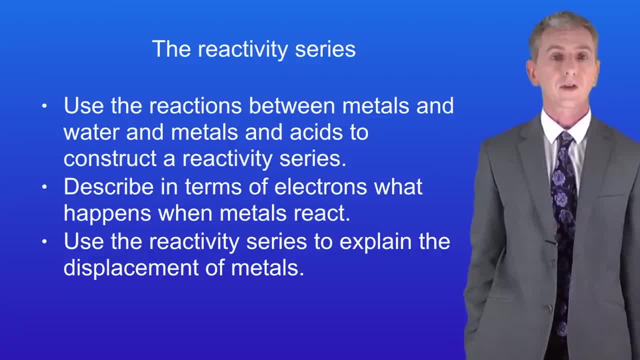 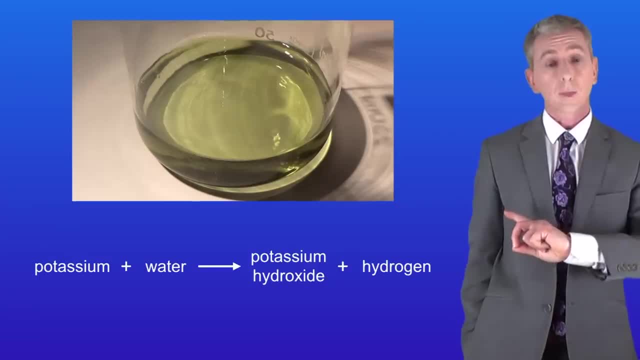 we're going to look at how we can use the reactivity series to explain the displacement of metals and acids. In a previous video we looked at how group 1 metals react with water, and I'm showing you here the reaction of potassium with water. As you can see, this is an extremely vigorous reaction When 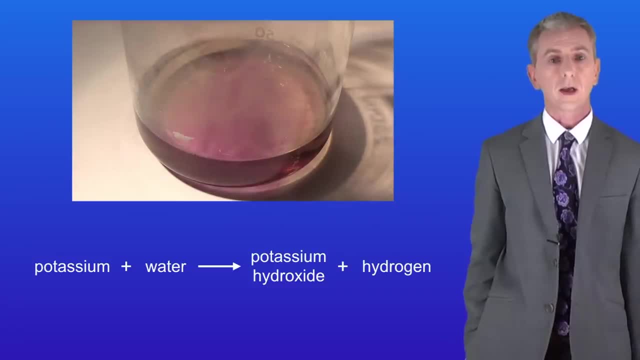 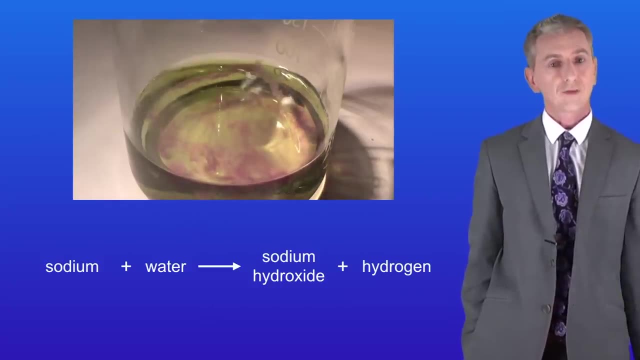 potassium reacts with water, we make the alkali potassium hydroxide and the gas hydrogen. Here's sodium reacting with water. As you can see, sodium reacts less rapidly with water than potassium. When sodium reacts with water, it produces the alkali sodium hydroxide and hydrogen gas. 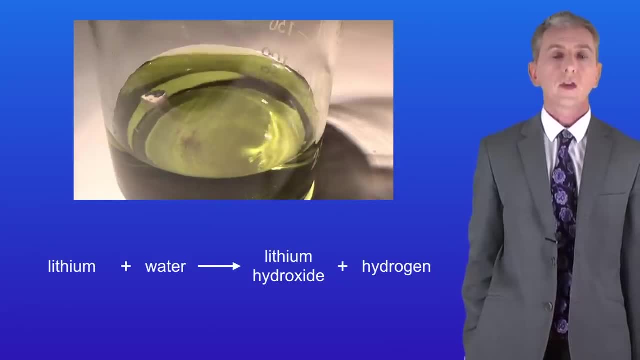 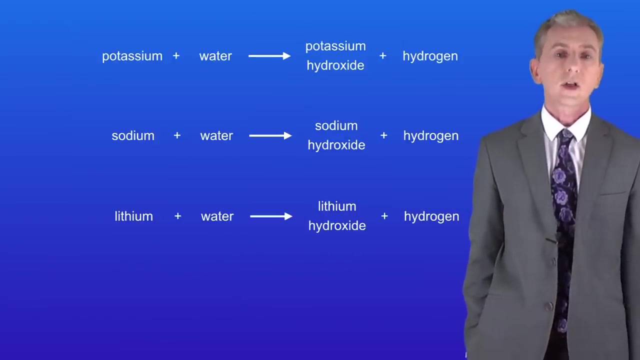 Finally, here's lithium reacting with water. Lithium reacts more slowly than either potassium or sodium. When lithium reacts with water, it produces the alkali lithium hydroxide and hydrogen gas. So I'm showing you here all of the reactions that we've seen so far As you can see reacting a metal. 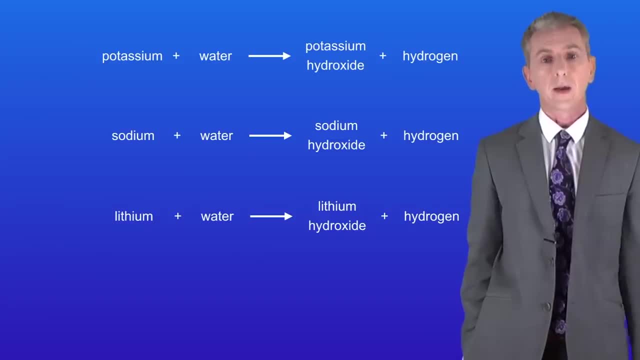 with water produces a metal hydroxide, which is an alkali and hydrogen gas. Calcium reacts with water in a very similar way. So I'm showing you that reaction here. We make calcium with water, potassium hydroxide and hydrogen gas. Calcium reacts fairly rapidly with water, but it's not as 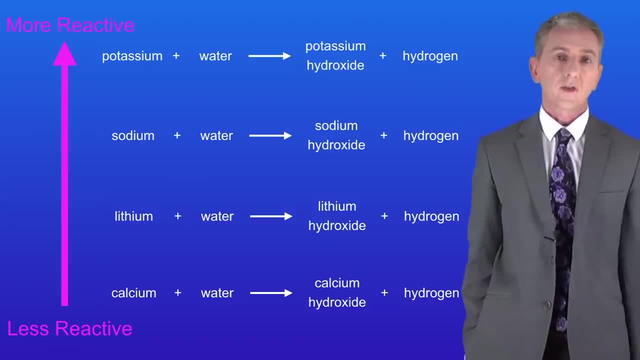 rapid as potassium, sodium or lithium. So, as you can see as we move down this list, the metals react less rapidly with water. By testing a whole range of different metals with water, we can work out the reactivity of the metals. I'm showing you the reactivities of the different metals with water. 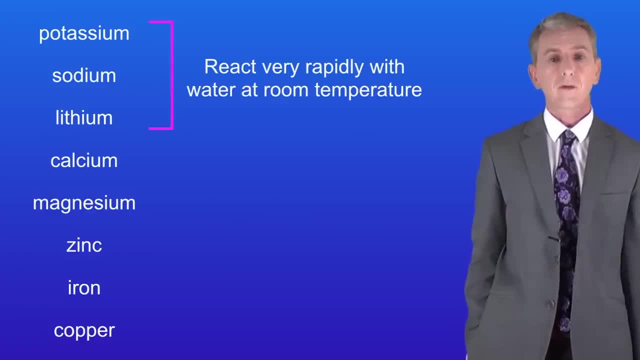 here. Potassium, sodium and lithium react very rapidly with water at room temperature. Calcium reacts very slowly with water at room temperature. Magnesium, zinc, iron and copper have got no reaction with water at room temperature, So we can use the reaction with water to determine the 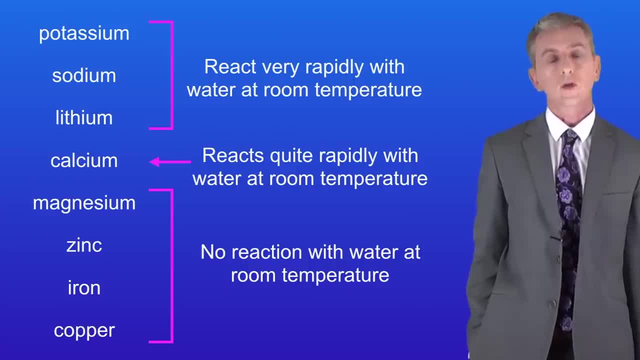 reactivity of potassium, sodium, lithium and calcium. But we cannot use water with magnesium, zinc, iron and copper, as they don't react with water. So if we want to compare the reactivity of these last four metals, then we need to react them with dilute acids We're going to look at. 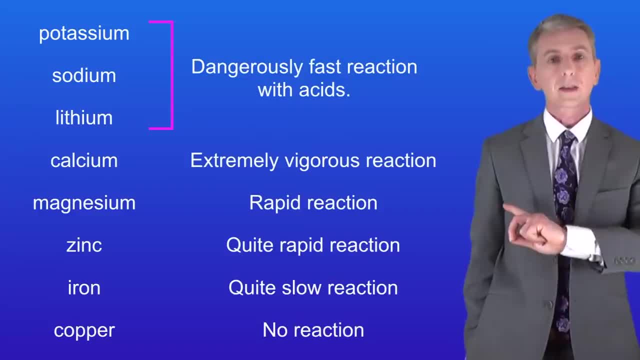 reactions of metals with acids in later videos. So here are the reactivities of the metals with dilute acids. Firstly, we'd never react potassium, sodium or lithium with acid, as they'd react too vigorously and that would be dangerous. Calcium reacts extremely vigorously with dilute acid, Magnesium reacts rapidly, Zinc reacts quite.